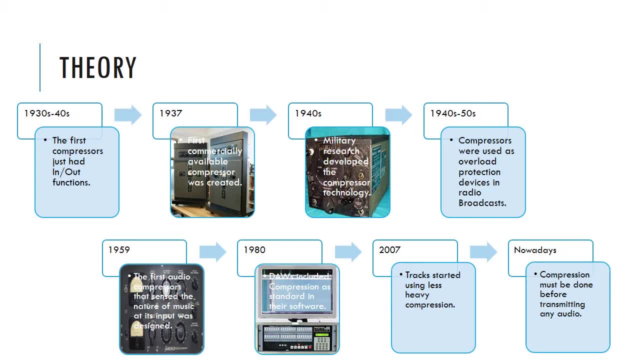 It was first started to control the volume of TV presenters with respect to audience clapping. At that time the compressor had just in-out functions. Then the first commercially available compressor was created in 1937.. After that the compressor technology developed due to military research. 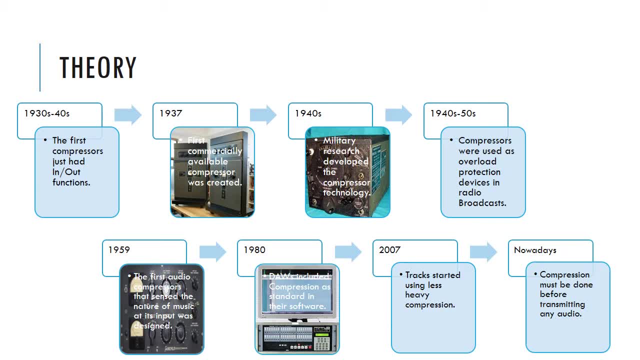 Compressors started to be used as overload protection devices in radio broadcasts In 1959, the American engineer designed the first audio compressor that sensed the nature of music at its input. In the 1980s, the digital audio workstation included compression as a software. 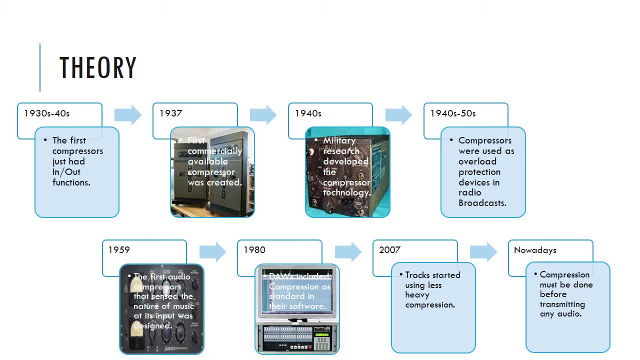 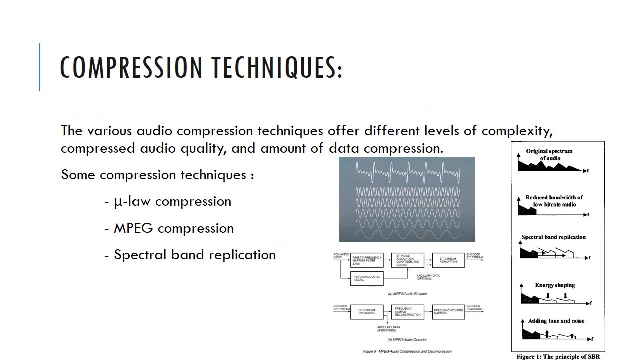 rather than needing compression racks, in 2007, tracks started using less heavy compression. nowadays, any audio that need to be transmitted or published need to be compressed first, and compression techniques are developed more. the various audio compression technique offer different level of complexity, compressed audio quality and amount of 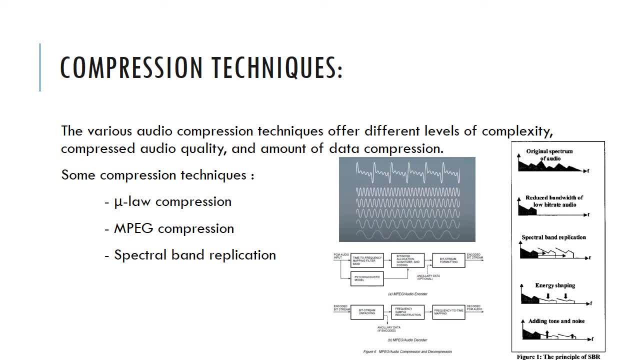 data compression. what follows is some audio compression techniques. the mu law quantization used in phone systems uses 8-bit of data to provide the dynamic range that normally requires 12 bit of PCM data. it is a low complexity, low compression technique and provides medium audio quality. the process of 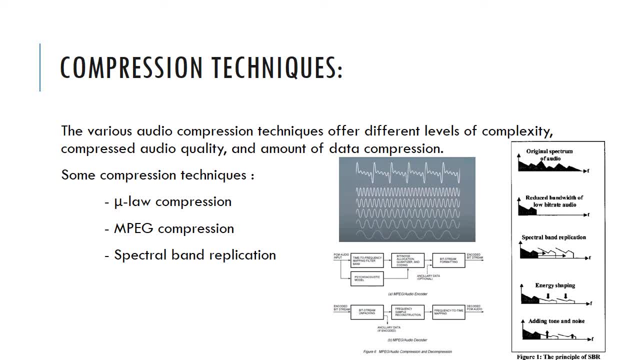 converting a computer file to mu law is a form of compression, since the amount of data that is needed per sample is reduced and the dynamic range of the sample is increased. the result is much, much less data with more information. to create a mu law data, the signal must be compressed and later. 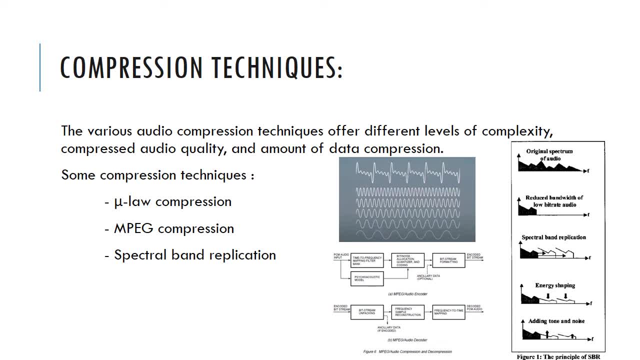 expressed expanded. this process is commonly referred to as compounding. the MPEG technique is a complex technique which offers a high compression and high quality audio. this standard utilizing technology compresses audio signal to make it audible to the human ear and removes the undesired signal introduced in the communication path, without assuming the nature of the audio source. 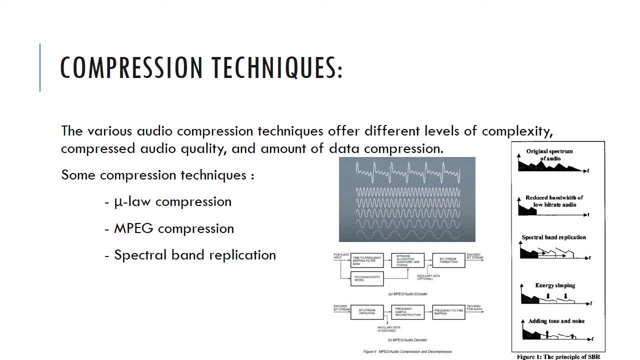 in MPEG technology, the fundamental parts of audio signals are maintained. MPEG technology also provides audio forward and reverse features by maintaining the bit stream of the audio signal and the sound of the audio signal. spectral band replication- SPR- is a technology to enhance audio or speech codecs, especially at low bit rates, and is based on harmonic redundancy in the